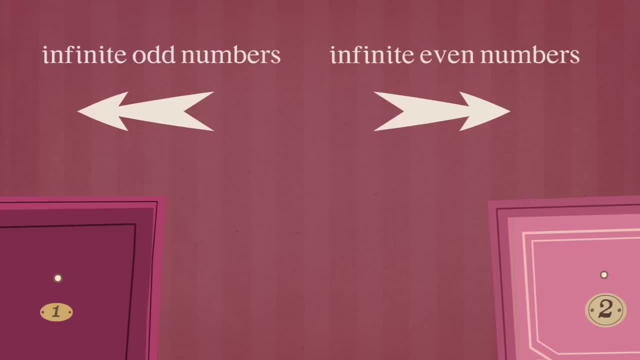 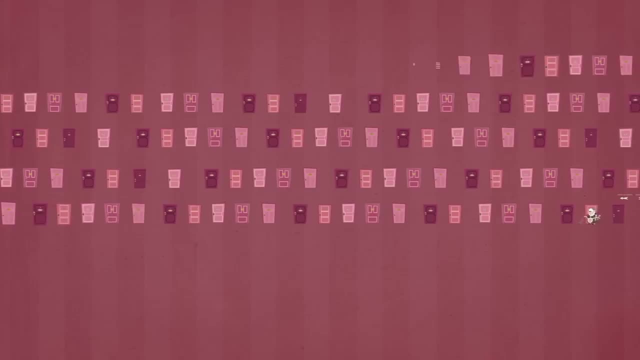 Each current guest moves from room number n to room number 2n, filling up only the infinite even-numbered rooms. By doing this, he has now emptied all of the infinitely many rooms, many odd-numbered rooms, which are then taken by the people filing off the infinite bus. 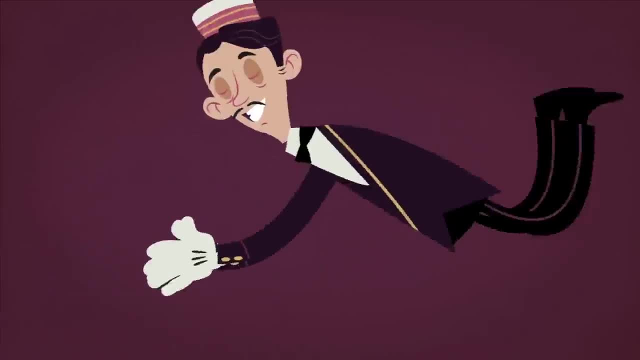 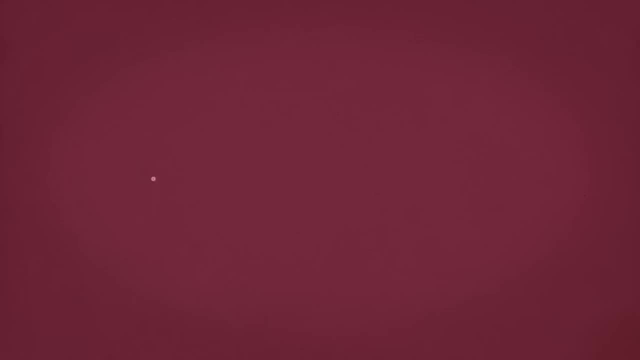 Everyone's happy and the hotel's business is booming more than ever. Well, actually it is booming exactly the same amount as ever, banking an infinite number of dollars a night. Word spreads about this incredible hotel. People pour in from far and wide. One night, 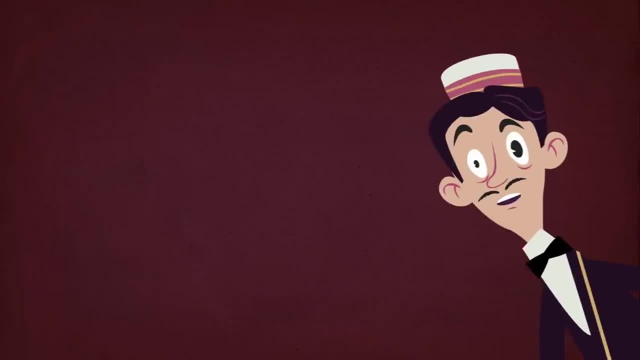 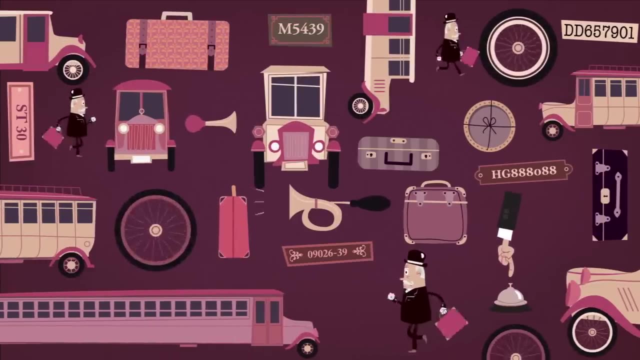 the unthinkable happens. The night manager looks outside and sees an infinite line of infinitely large buses, each with a countably infinite number of passengers. What can he do If he cannot find rooms for them? the hotel will lose out on an infinite amount of money. 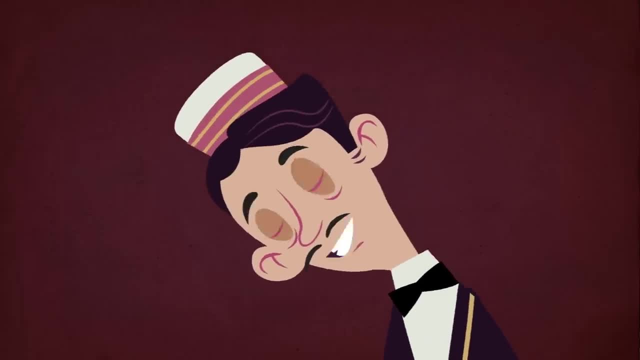 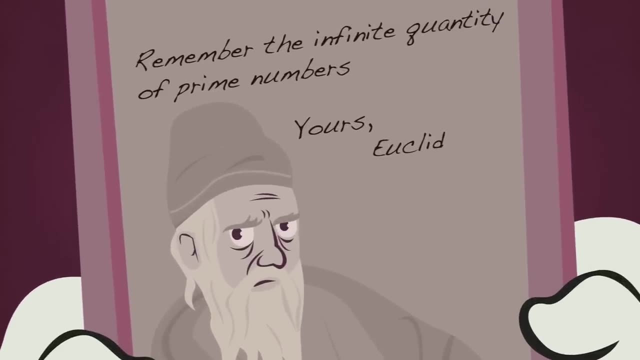 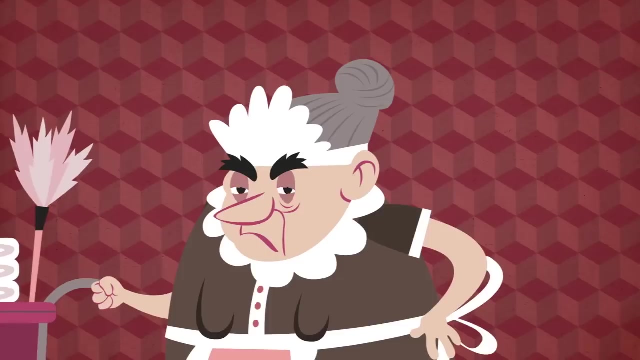 and he will surely lose his job. Luckily he remembers that around the year 300 BCE, Euclid proved that there is an infinite quantity of prime numbers. So to accomplish this seemingly impossible task of finding infinite beds for infinite buses, of infinite weary travelers. 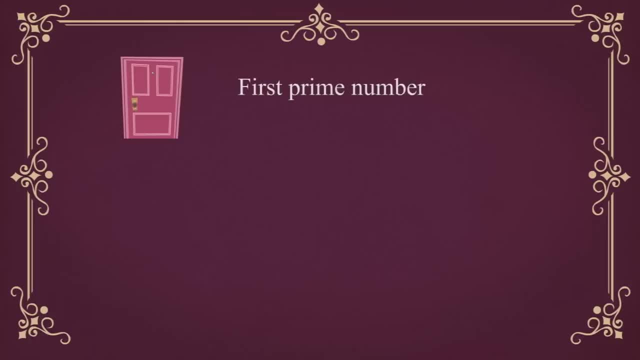 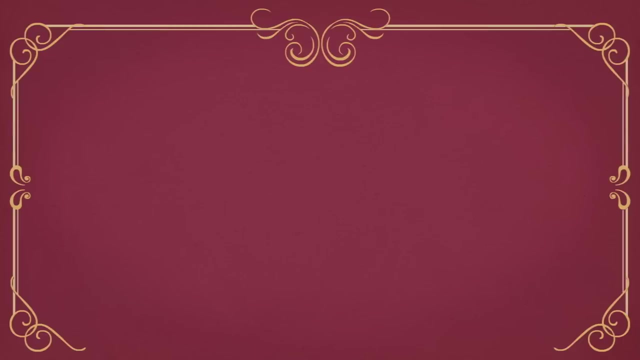 the night manager assigns every current guest to the first prime number two raised to the power of their current room number. So the current occupant of room number seven goes to room number two, to the seventh power, which is room 128.. The night manager then takes the people on the first of. 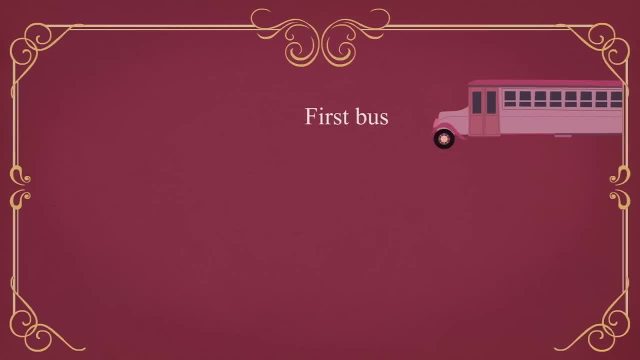 the infinite buses and assigns them to the room number of the next prime three raised to the power of their seat number on the bus. So the person in seat number seven on the first bus goes to room number three, to the seventh power or room number 2,187.. This continues for all of the 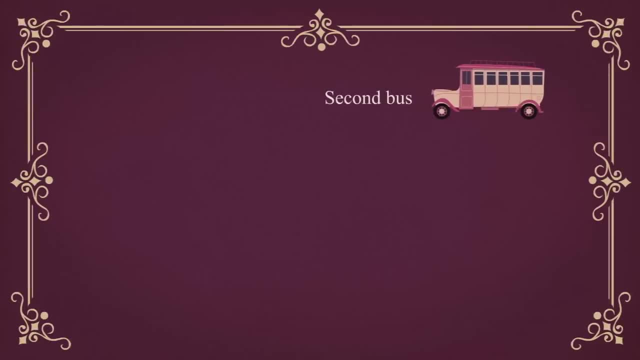 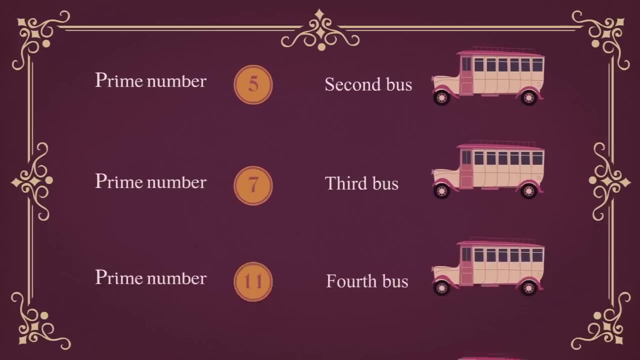 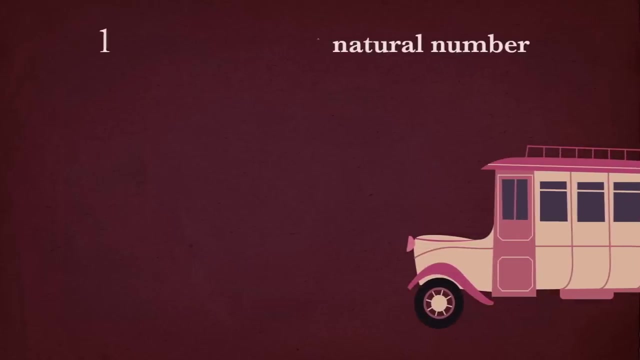 first bus, The passengers on the second bus are assigned powers of the next prime five, The following bus: powers of seven. Each bus follows powers of 11,. powers of 13,. powers of 17,, etc. Since each of these numbers only has one and the natural number, powers of their prime number base. 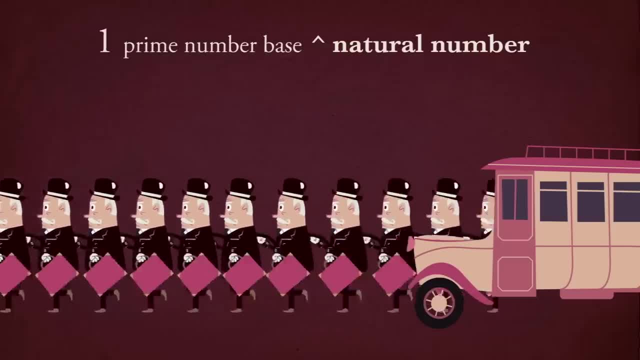 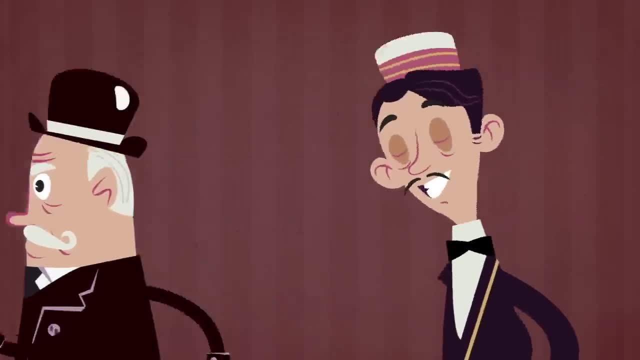 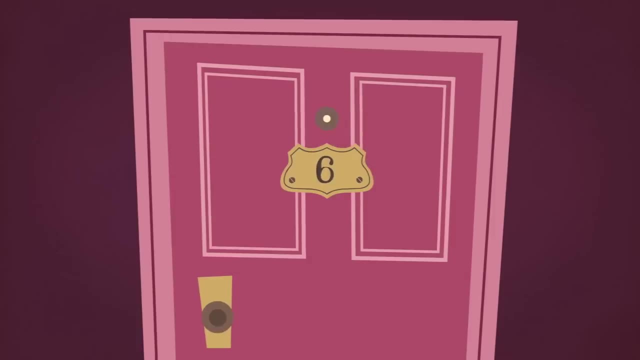 as factors. there are no overlapping room numbers. All the bus' passengers fan out into rooms using unique room assignment schemes based on unique prime numbers. In this way, the night manager can accommodate every passenger on every bus, although there will be many rooms that go unfilled, like room six, since six is not a power of any. 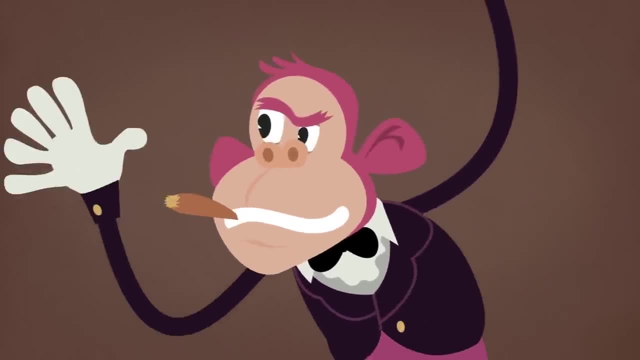 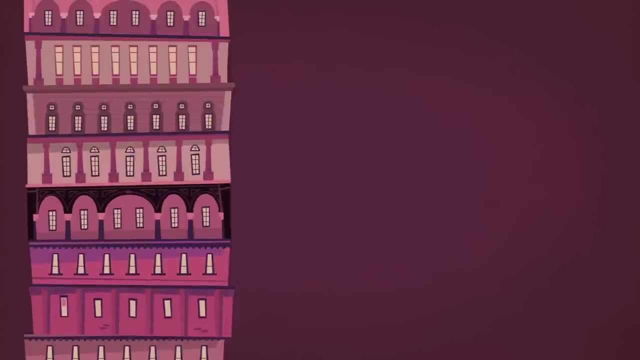 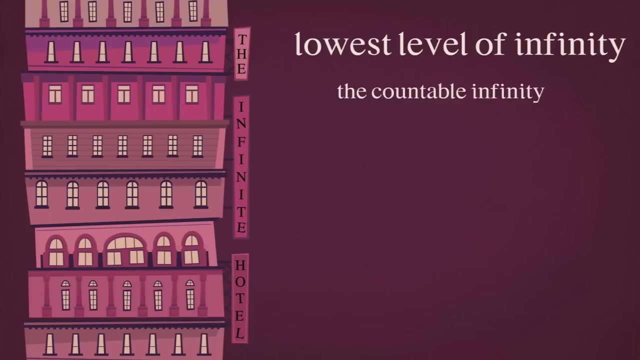 prime number. Luckily his bosses weren't very good in math, so his job is safe. The night manager's strategies are only possible because, while the infinite hotel is certainly a logistic nightmare, it only deals with the lowest level of infinity, namely the countable infinity of the 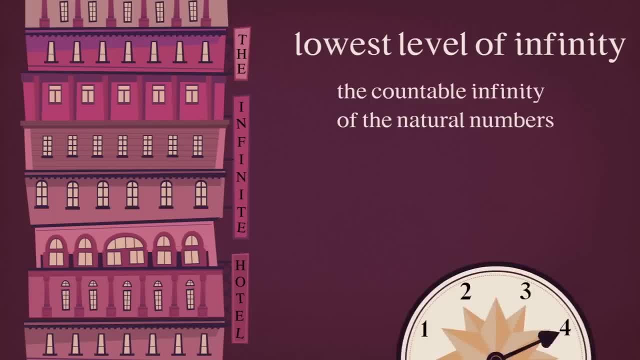 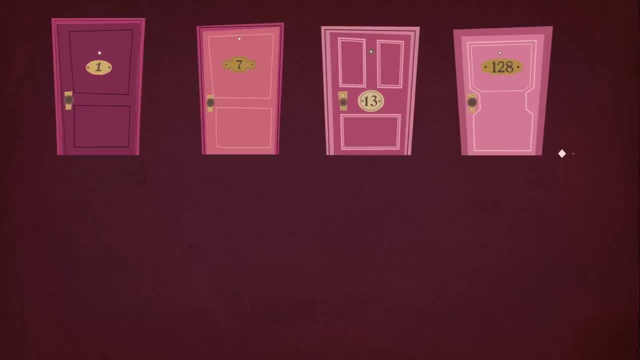 natural numbers: one, two, three, four and so on. Georg Cantor called this level of infinity aleph zero. We use natural numbers for the room numbers as well as the seat numbers on the buses If we were dealing with higher orders of infinity such as that of the real numbers. 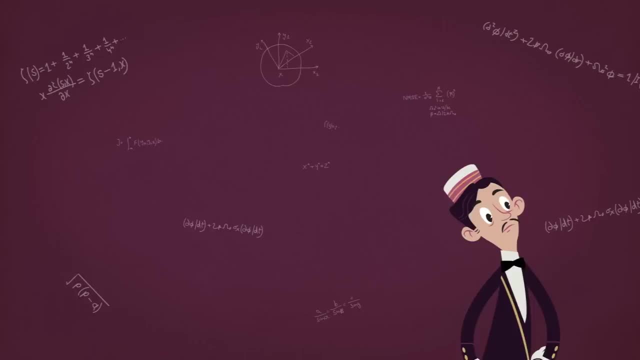 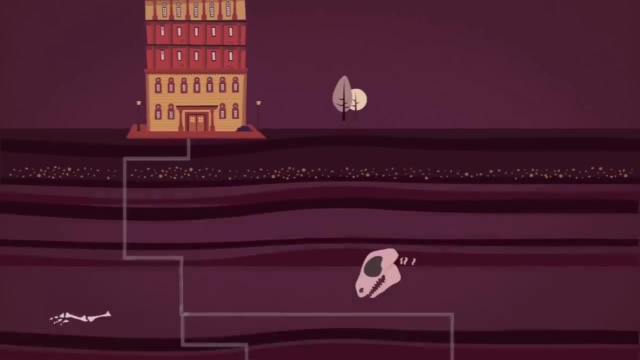 these structured strategies would no longer be possible as we have no way to systematically calculate the number of rooms in the room, The real number. infinite hotel has negative number rooms in the basement- fractional rooms, so the guy in room one-half always suspects he has less. 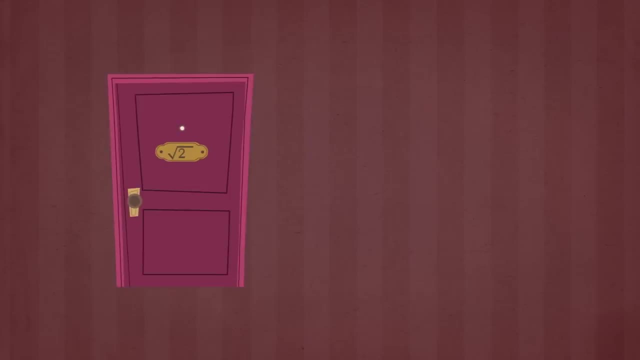 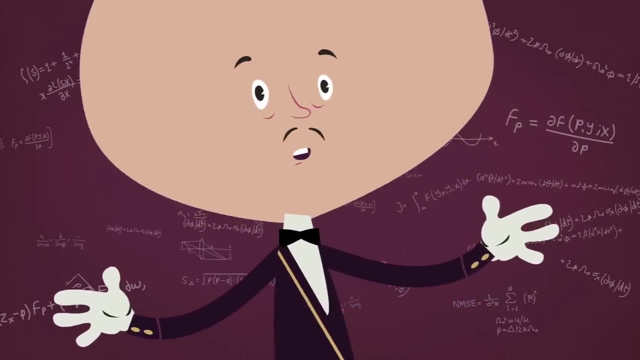 room than the guy in room one. square root rooms like room radical two and room pi, where the guests expect free dessert. What self-respecting night manager would ever want to work there, even for an infinite salary, But over at Hilbert's infinite hotel where there's never any vacancy? 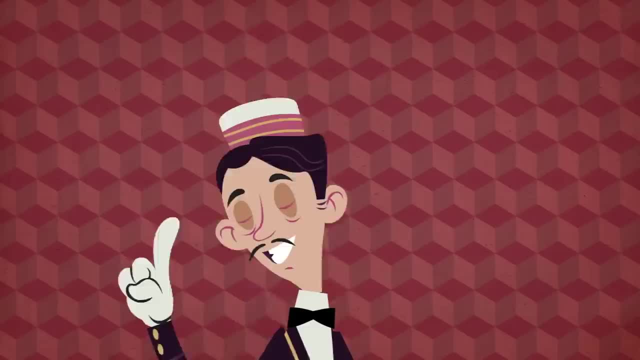 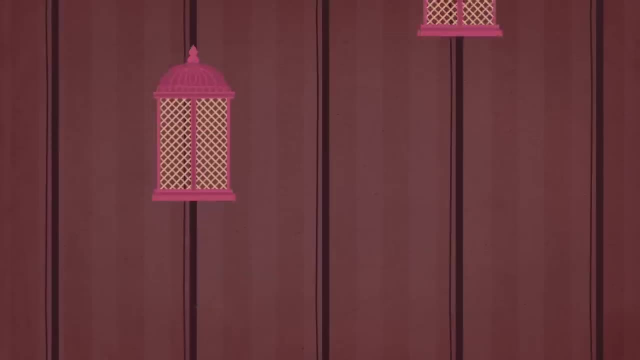 and always room for more. the scenarios faced by the infinite hotel are not the same as the ever diligent and maybe too hospitable night manager serve to remind us of just how hard it is for our relatively finite minds to grasp a concept as large as infinity. Maybe you can help tackle. 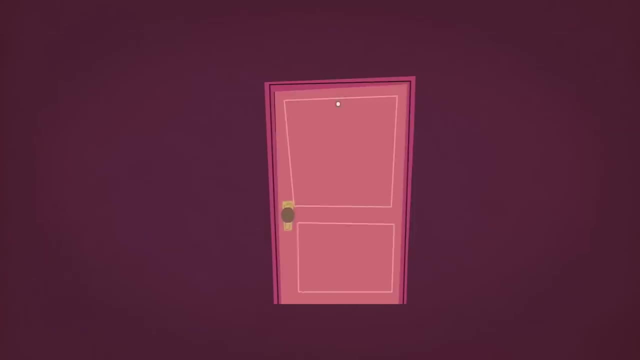 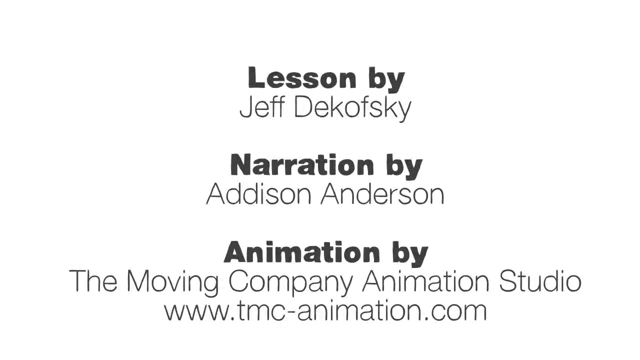 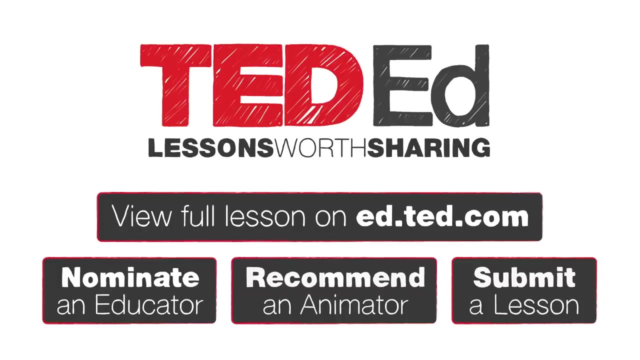 these problems after a good night's sleep, but honestly, we might need you to change rooms at 2am. Thank you for watching.